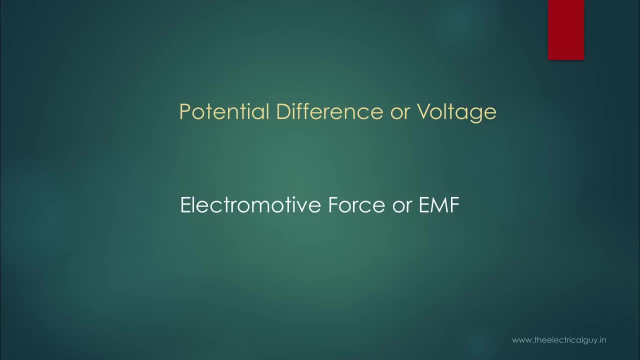 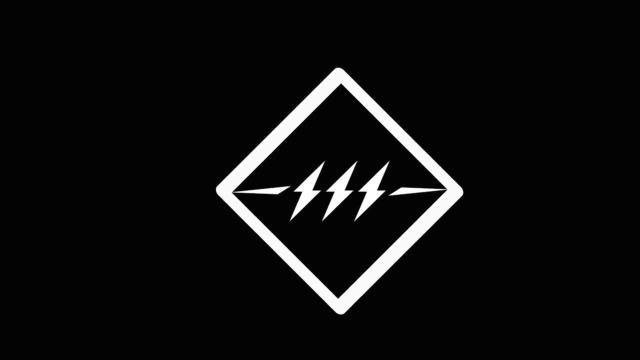 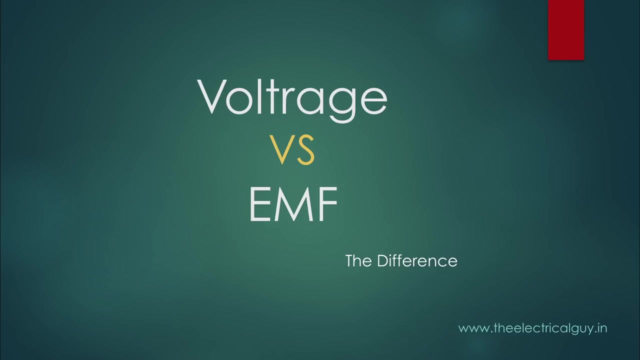 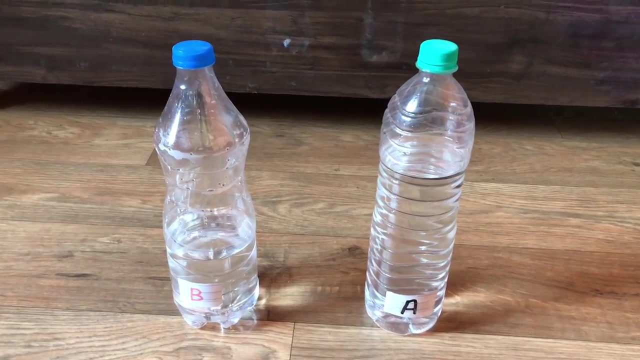 and electromotive force. So to know the details and the difference between these two, you need to watch the video To understand the difference between potential difference, or voltage, and emf. let's do an experiment Here. I have two bottles filled with water, As you can see, 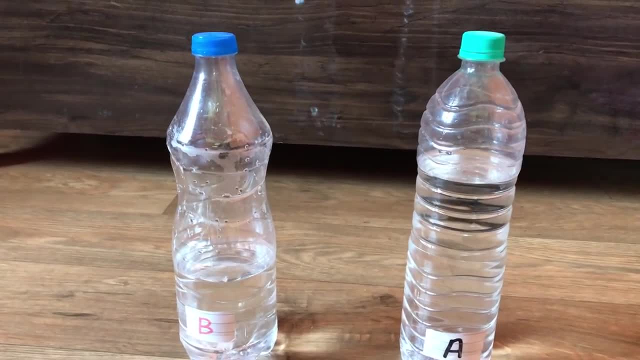 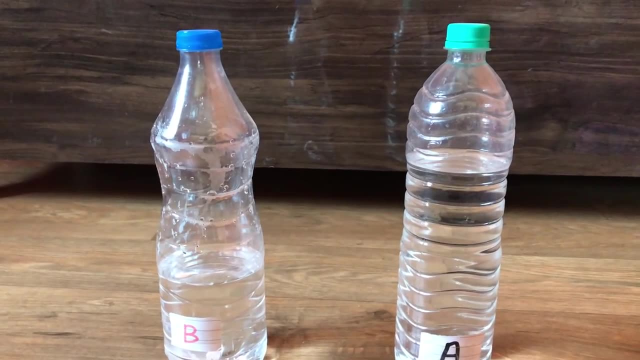 bottle A is filled with water above center line of the bottle and in bottle B water is filled below center line. In technical language I would say bottle A is having electric potential of 10V and bottle B is having electric potential of 4V. Now if I connect a small pipe between these two bottles, then what will happen? 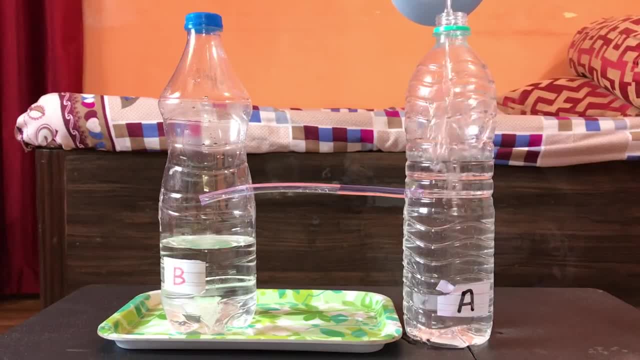 Let's check that out. So, as you can see, after connecting a pipe between these two bottles, water has started flowing from bottle A to bottle B, that is, from higher potential to lower potential. Water is flowing because there is a difference in water level of both. 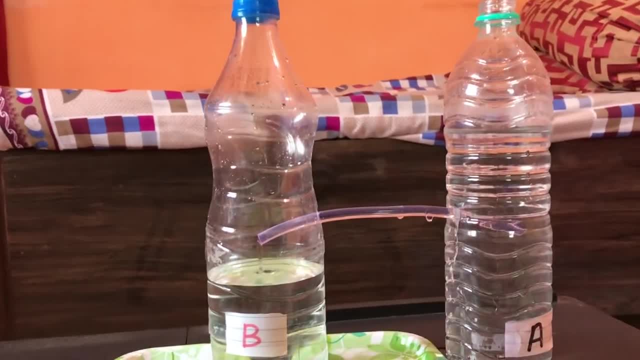 the bottle A and the bottle B, which is the same. So, if you connect a small pipe between these two bottles, then what will happen? So, as you can see, after connecting a pipe between these two bottles, bottles Water will now continue to flow until water level of both the bottles becomes same. 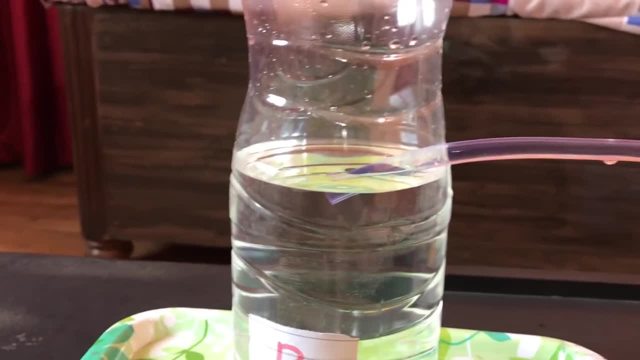 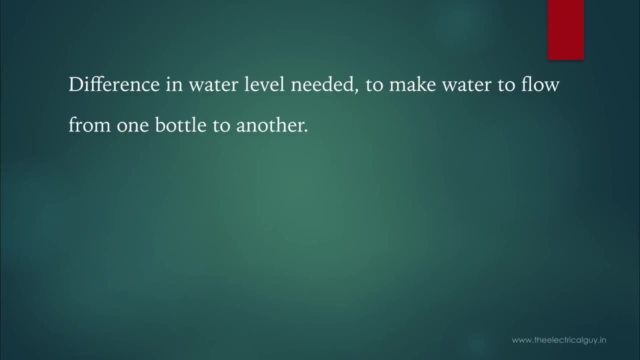 Here you can see, water is not flowing as the level of both the bottles are now equal. So what we understood- difference in water level- needed to make water to flow from one bottle to another. In technical language, I would call this difference in water level as potential difference or voltage. 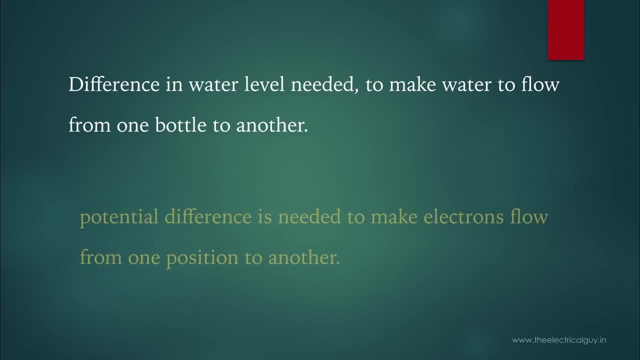 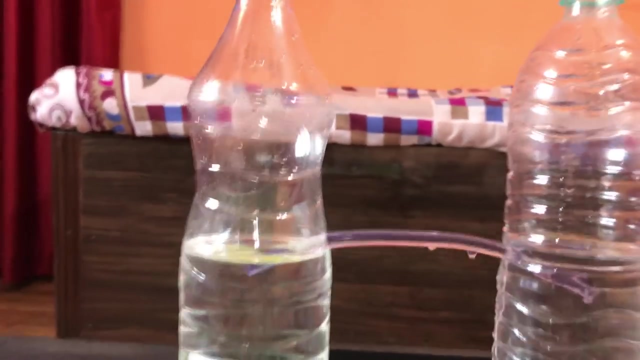 So now I can modify my sentence, as potential difference is needed to make electrons flow from one position to another. So we are now clear about the potential difference or voltage. Potential difference or voltage is required to make electrons flow from one position to another. Now let's get back to our experiment. As you can see, water level of both the bottles are: 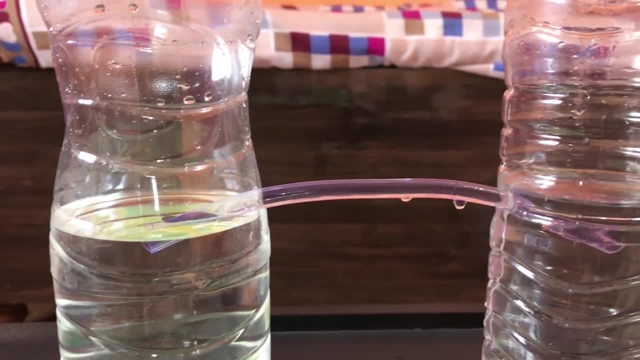 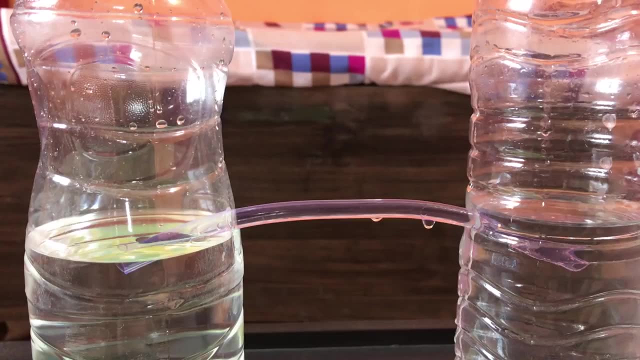 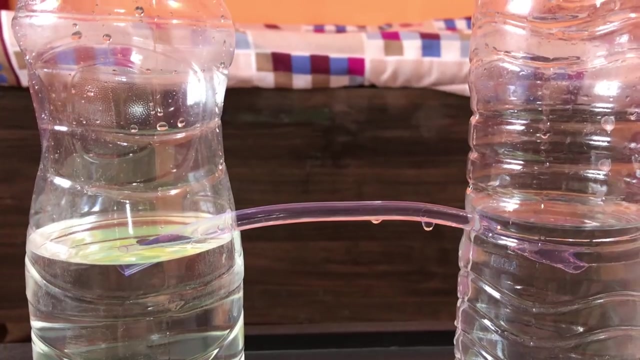 equal and hence no water is flowing. But what if we need continuous flow of water? To do that, let's say I connected a device which will again create the difference in water level of both the bottles. I cannot show you that here, so let's watch it graphically Here: I have connected. 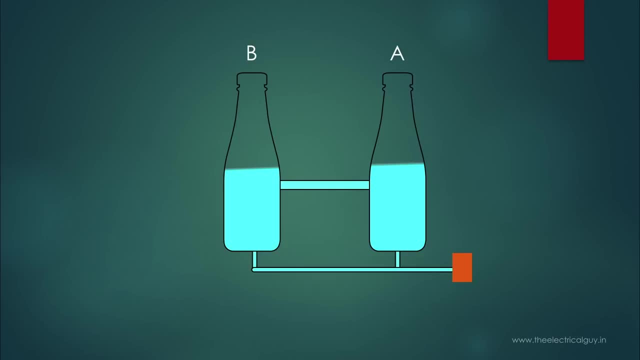 a device which will create difference in water level of both the bottles again, and now water will again start flowing Again. water level of both the bottles will become equal. so our device will again create the difference in water level and water will flow again. Now this process will 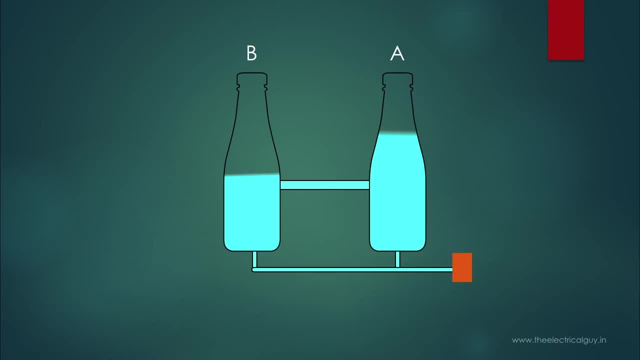 keep on repeating and we will get continuous flow of water. In technical language, I would say our device is maintaining the potential difference, that is, difference in water levels, and once it starts maintaining the potential difference, I can say it has developed the electromotive force, or EMF in short. So what we understood, EMF is needed to maintain the potential difference. 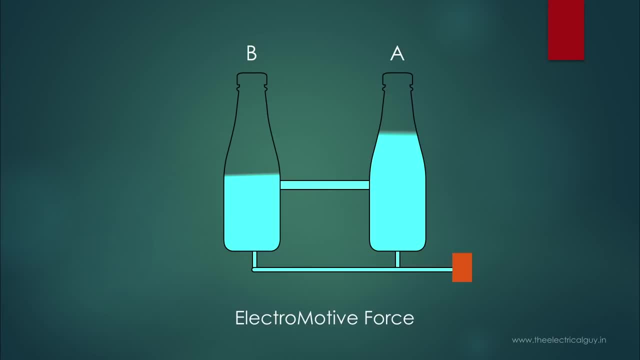 because of the name, Some people will think that EMF is a force. but it's not a force. it's an energy supplied by a device like a battery. So potential difference causes electrons to flow from one position to another, while E, M, F maintains the potential difference. To understand these terms more: 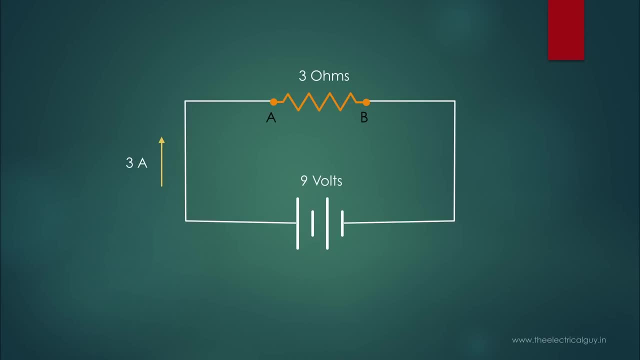 clearly. let's do one more experiment Here. I have a battery of 9v and a resistance of 3 ohm. I have connected this resistance with battery using a connecting wire, And current going through this circuit is 3A. Using Ohm's law, we can calculate that Our battery is. 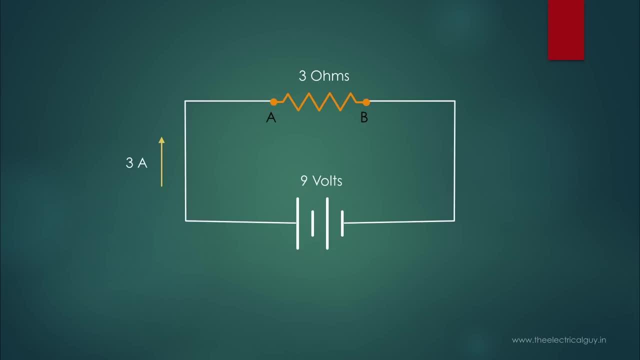 having emf of 9V, which means battery is supplying 9 joules of energy to each coulomb. Well, if you would like to know in detail about the concept of voltage and emf, you can watch my video on that. You will get link for that video down in the description. Journey of 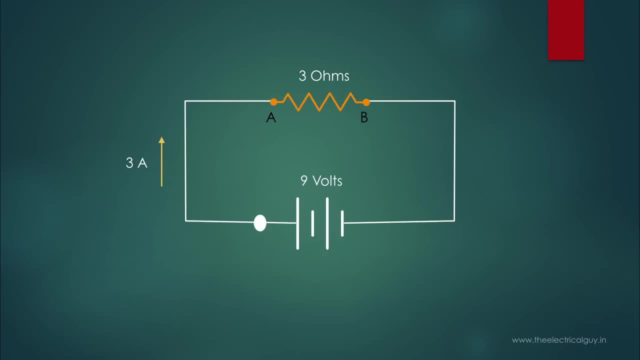 each coulomb starts with the positive terminal of battery and then it reaches to the point A. To travel from point A to point B, each coulomb will require 9 joules of energy. The energy used by each coulomb in moving from point A to point B is known as potential difference. 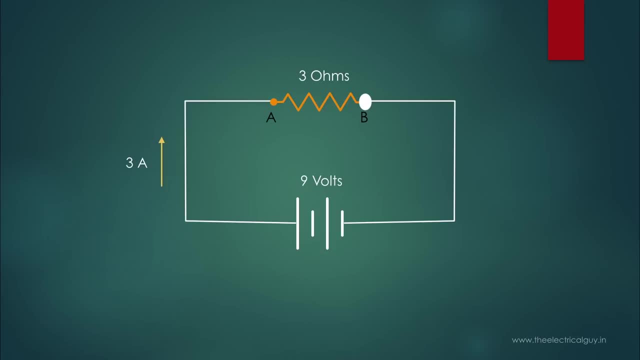 between those two points. Thus, in our example, potential difference between point A to point B is 9V. You can calculate that using Ohm's law. This potential difference between point A and point B is sometimes also called as voltage drop. These voltage drop will cause heat from resistance After losing most of